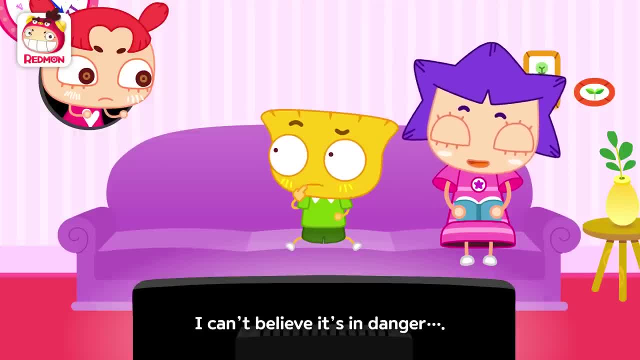 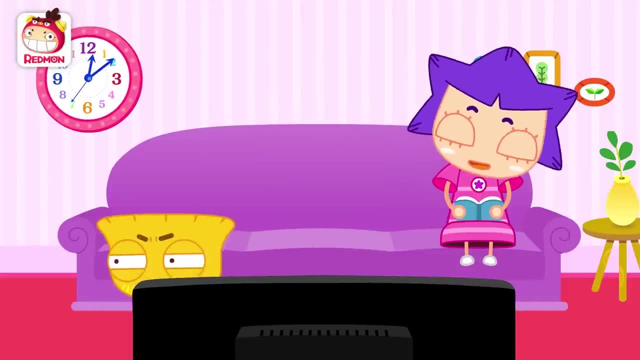 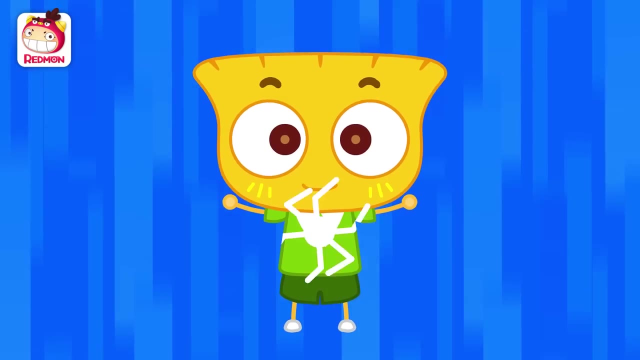 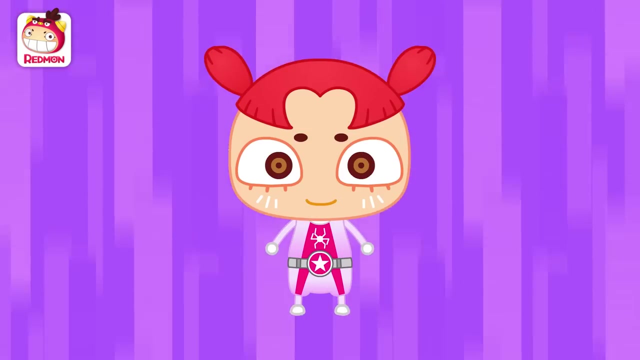 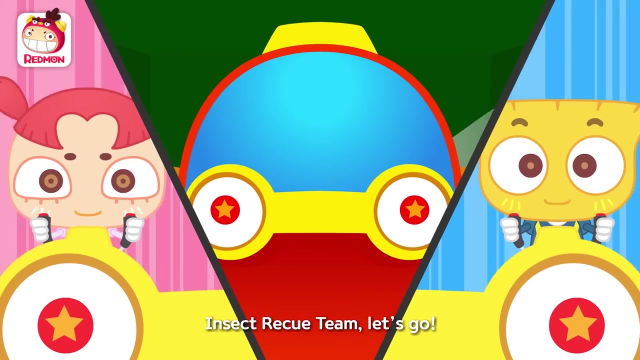 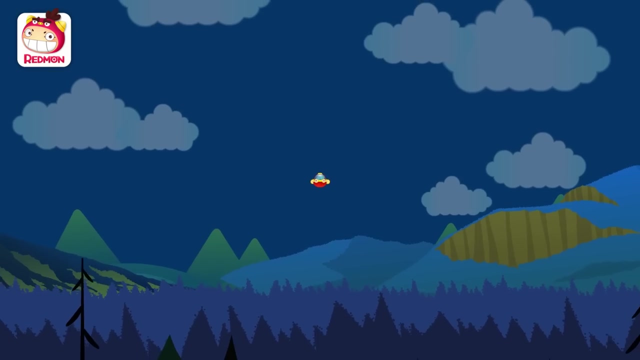 Tadpoles and even frogs. I can't believe it's in danger. Stop talking, Let's move. Okay, Mary, Insect rescue team, Let's go. Let's go Find the male giant water bugs. They must be protecting the eggs. 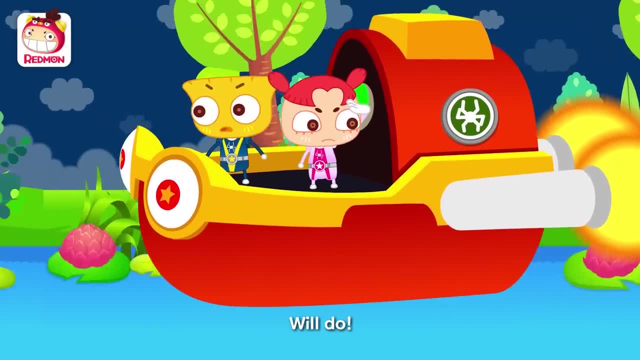 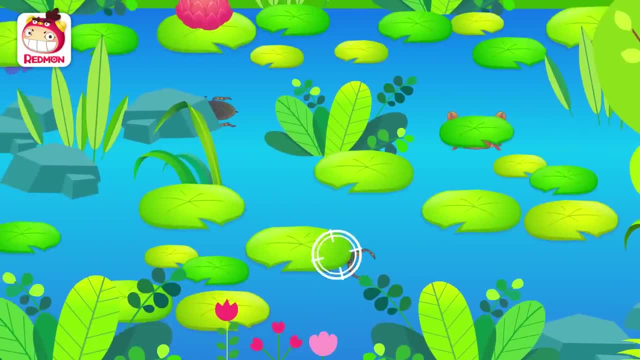 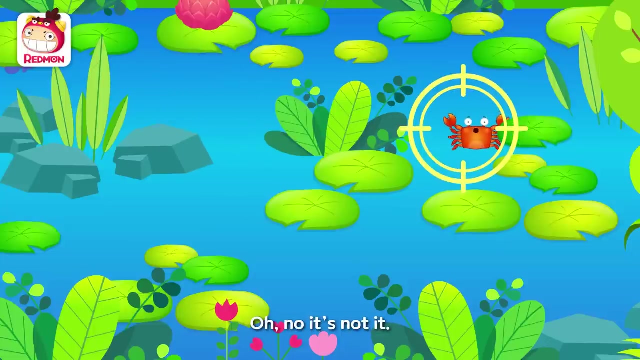 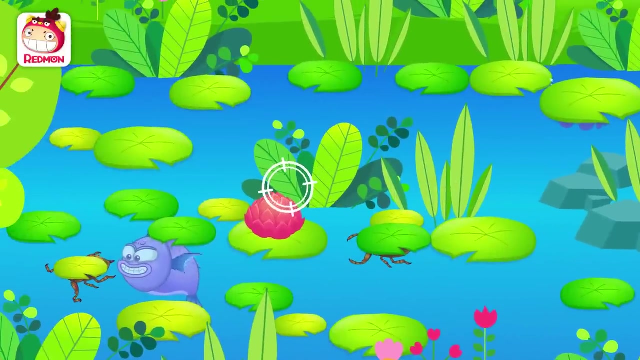 Male giant water bugs protect the eggs Will do? I found one. I found it. I found one too. Oh no, it's not. it Look closely. I found it Over there. Oh goodness, Oh goodness. 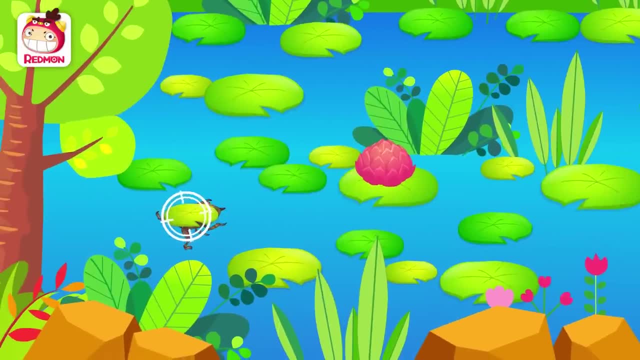 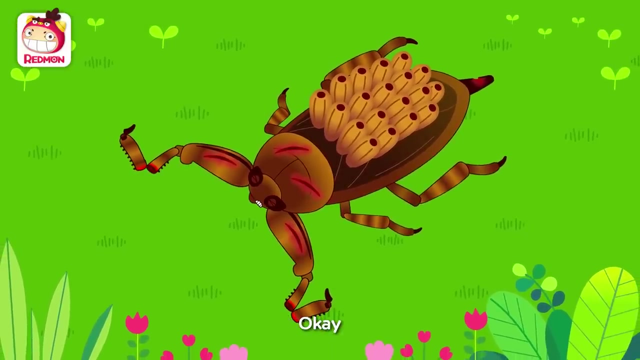 It's here. I found one, That's all. Good job, Robby. He got injured while protecting the eggs. Let's treat him now. Okay, I'll disinfect the wounds. I'll disinfect the wounds. Okay, It's alright. T Nelson. 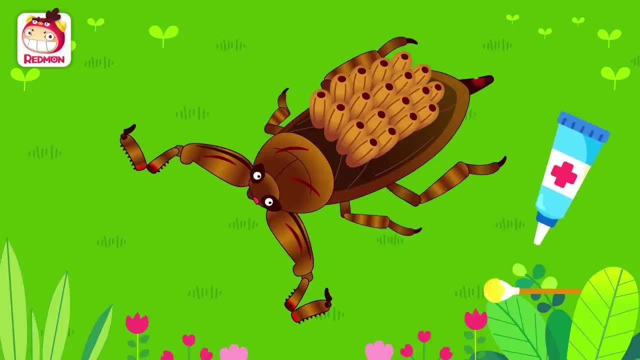 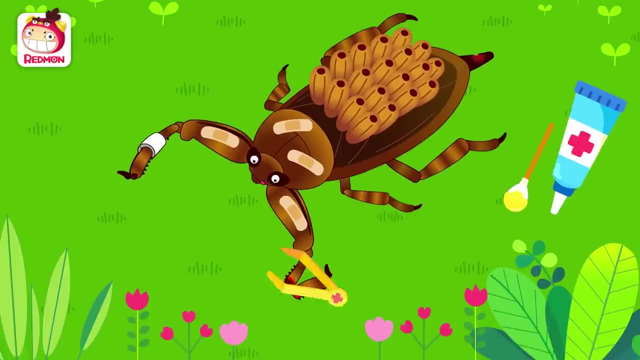 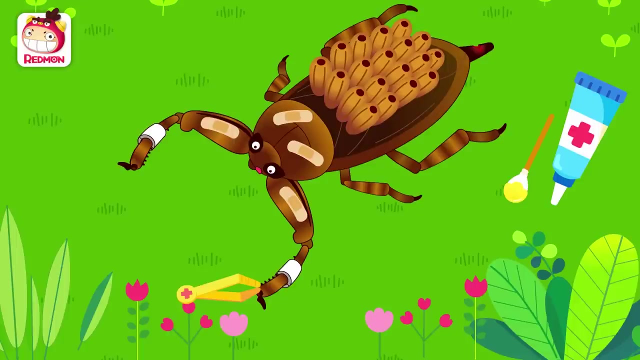 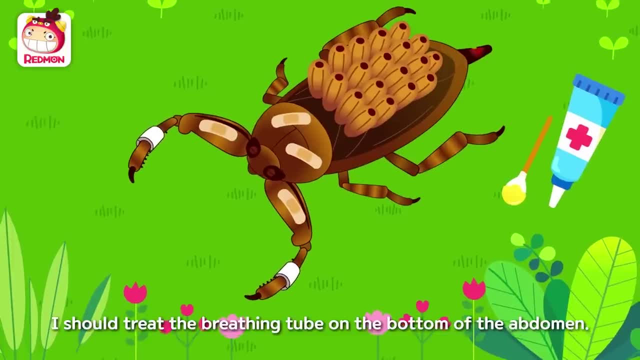 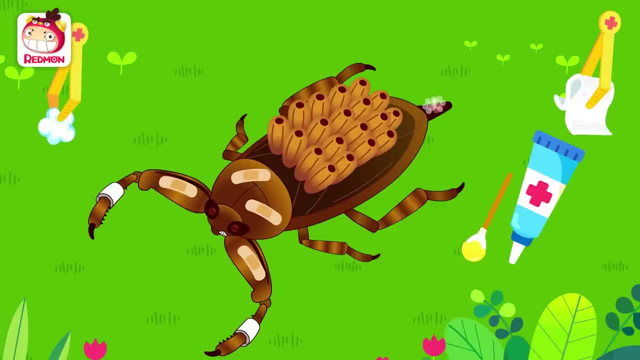 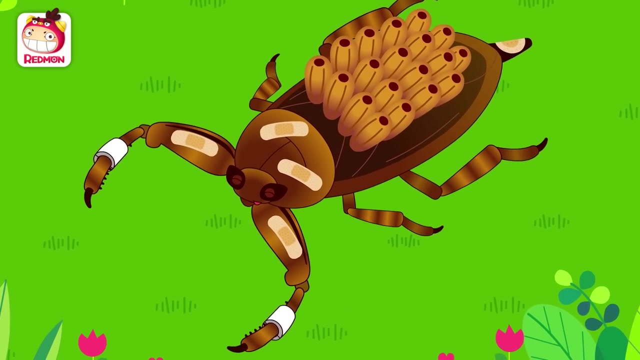 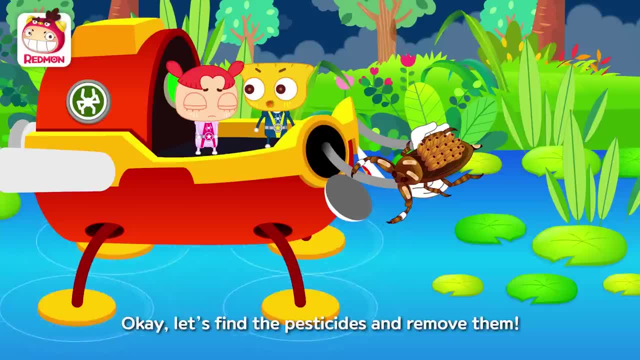 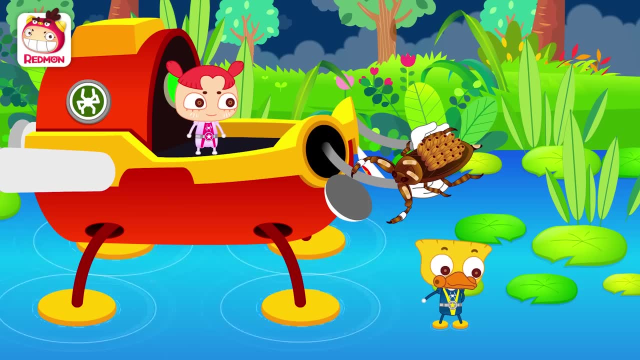 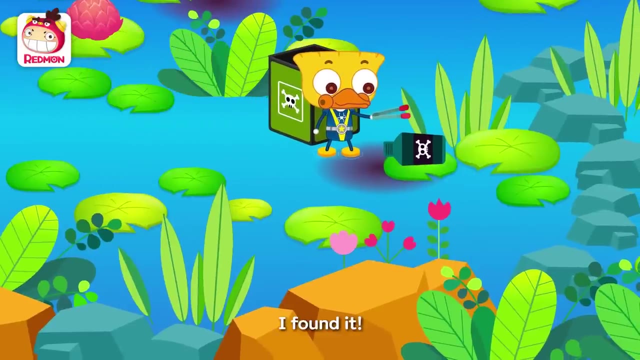 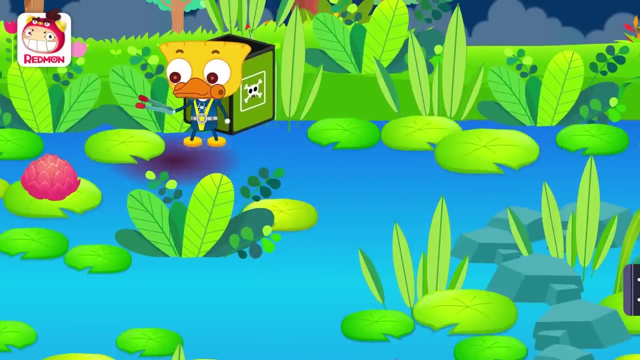 Robbie, the population of giant water bug is decreasing Because of pesticide use and water pollution. Okay, let's find the pesticides and remove them. Okay, let's do it. Okay, let's do it. I found it, It's here. 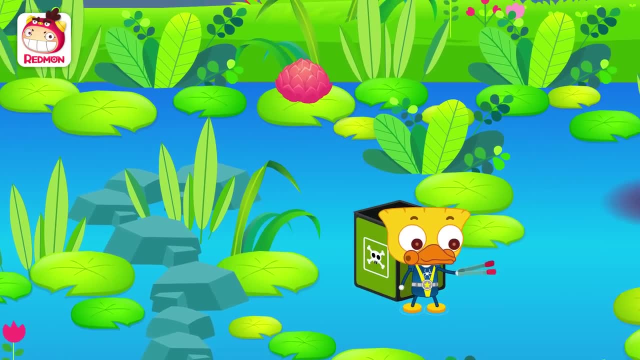 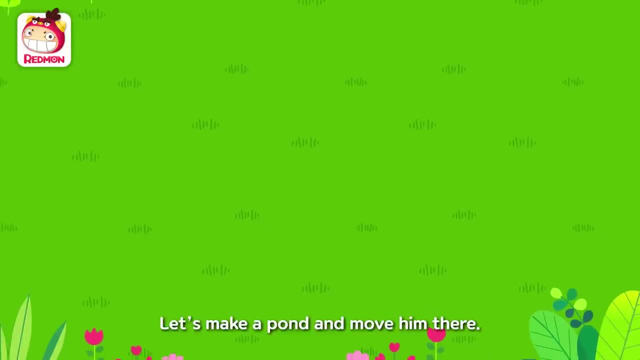 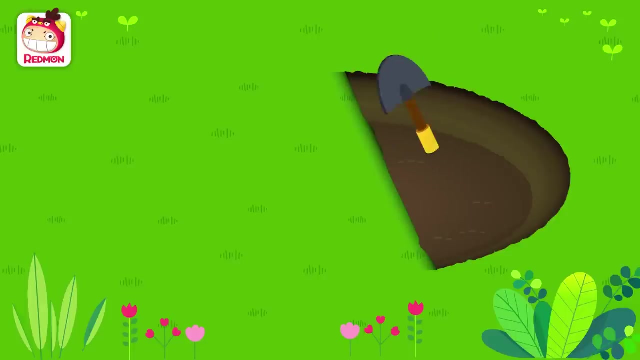 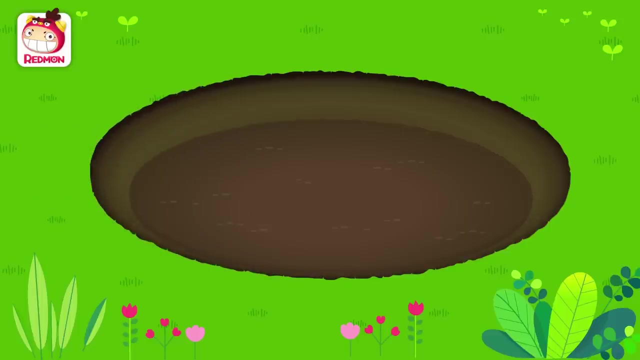 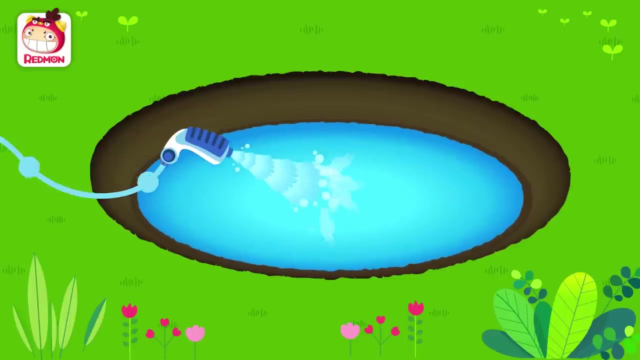 I found it again. I found it again. It's here. Phew, I'm finished. Phew, I'm finished. Phew, I'm finished. Let's make a pond and move him there. Okay, Mary, let's add a lot of water plants.